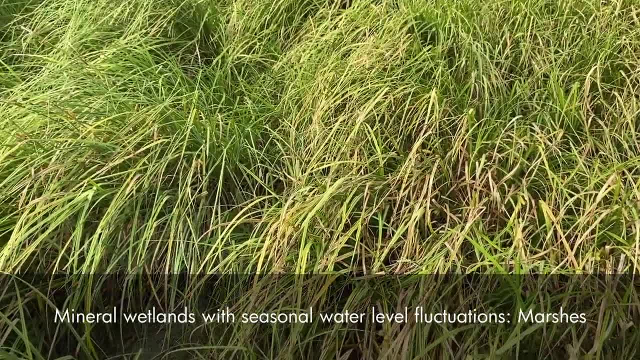 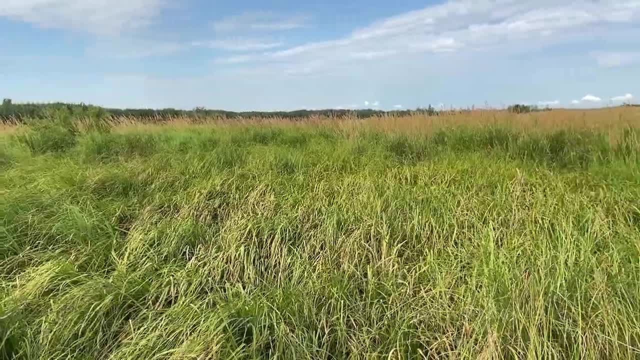 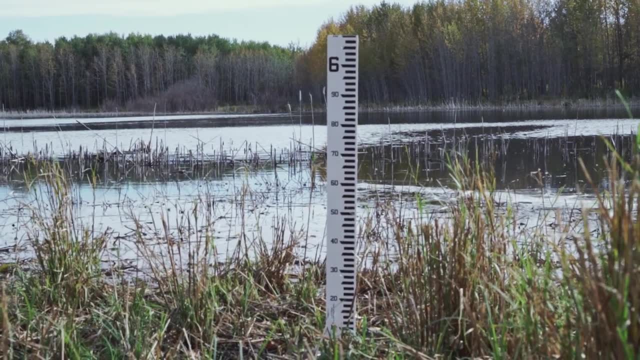 rainfall. Often these wetlands are dry by midsummer and difficult to identify. As a result, human disturbance impacts may be difficult to mitigate or avoid. There are several hydrology field methods that can be used to measure wetland water levels and water movement, such as monitoring wells and staff gauges. 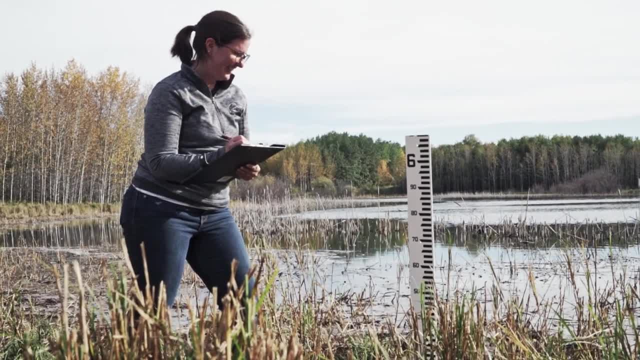 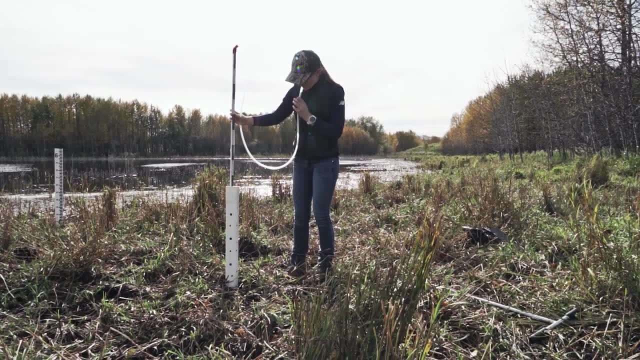 Staff gauges are used to quickly relay the depth of standing water at a single measurement point. Monitoring wells are used when surface water is not present. as they are installed below the ground, surface Water level measurements can be completed regularly by field crews, or data loggers can be deployed within. 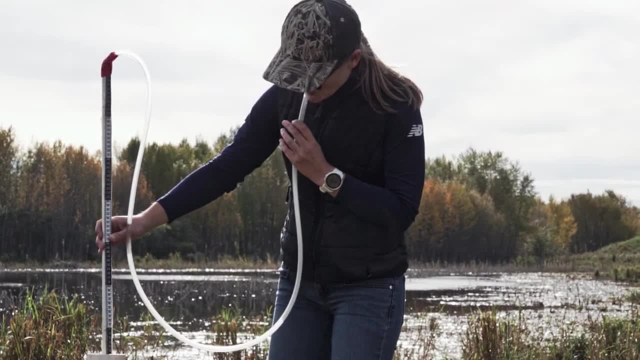 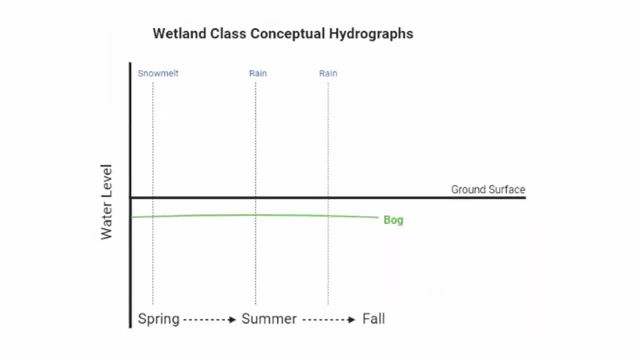 monitoring wells to take continuous water level measurements. The resulting data is plotted on a wetland hydrograph. This illustrates how each wetland class has a different season water level regime. Peatland, bogs and fens experience little water level fluctuation, with a consistently high. 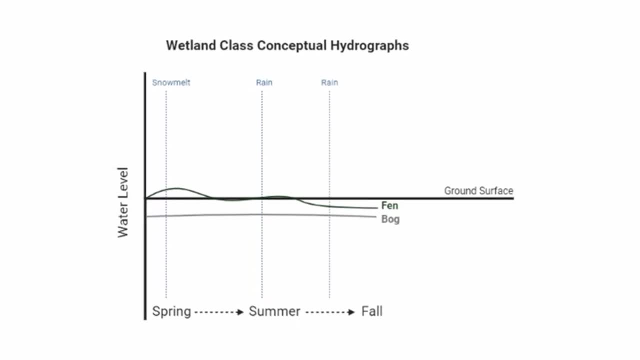 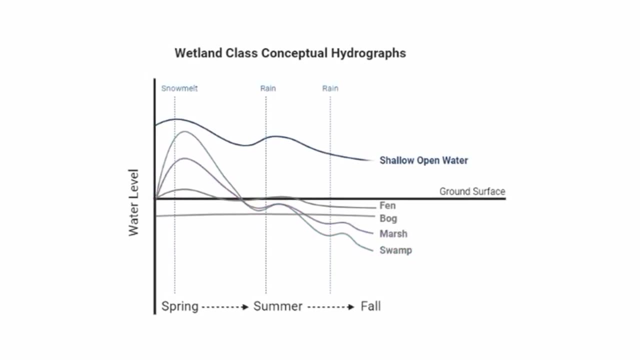 water table, residing just below or at the peat surface. In swamps, marshes and some shallow open water wetlands, the water level fluctuates considerably over the growing season, producing a flashier hydrograph. Temporary and seasonal systems will typically be dry by midsummer. 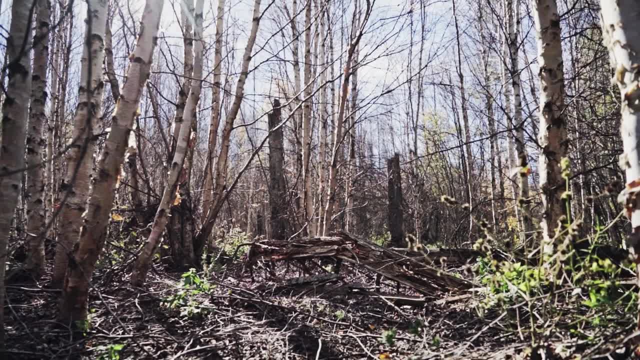 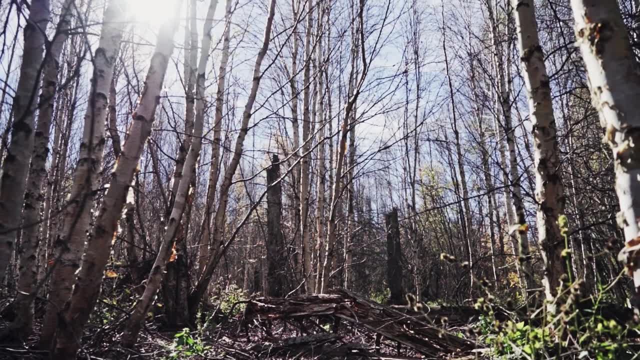 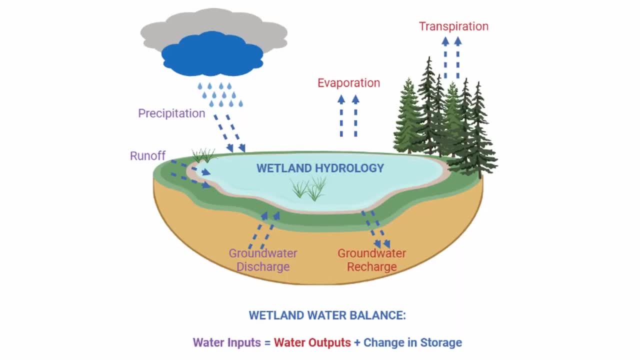 Monitoring the wetland water level is one tool in our toolbox for understanding wetland hydrology. If you've noticed that the area is getting wetter over time, with tree dieback, that might be the result of more frequent or severe flooding. these measurements can validate your observations. Another aspect of wetland: 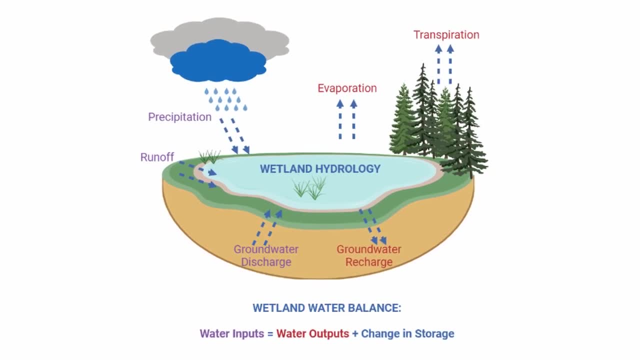 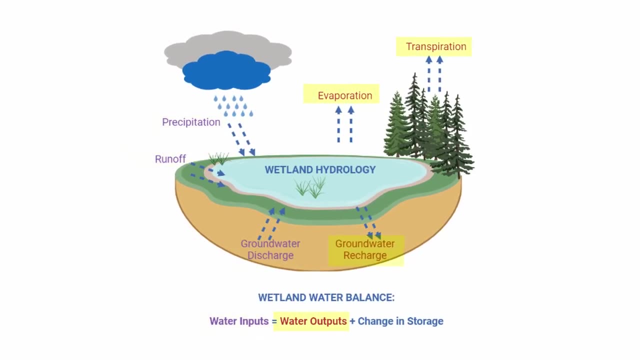 hydrology that is important to understand is how much water enters and leaves a wetland. A hydrologist might calculate a wetland water balance where water inputs equal water outputs. This can also tell us if a wetland is consistently gaining or losing water, which has implications for site management. 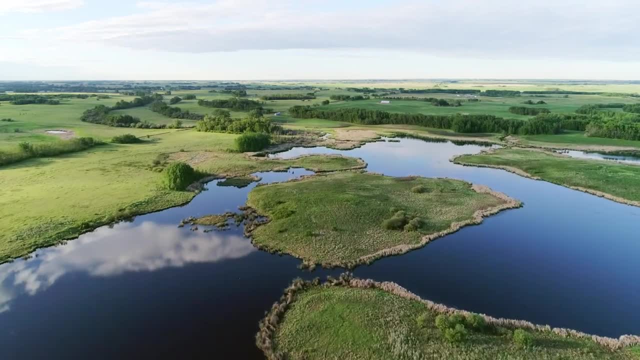 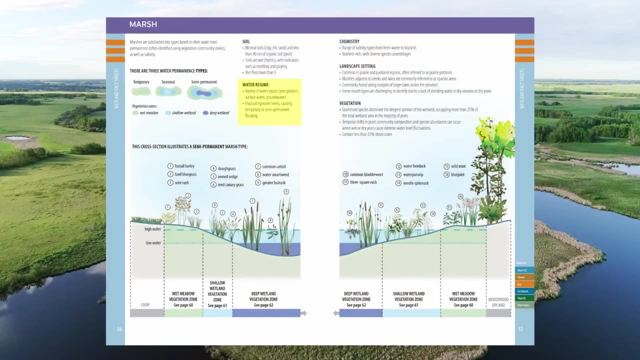 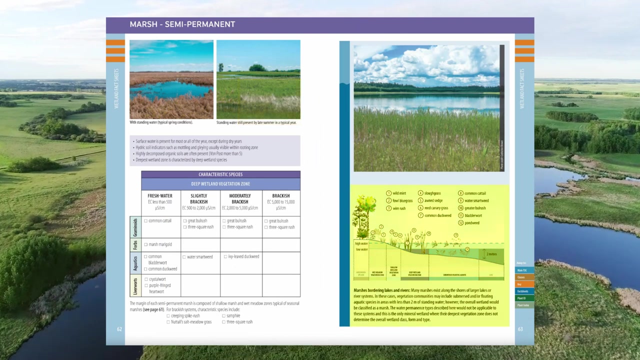 Some wetlands, such as those common in the prairie pothole region, exist in small, isolated watersheds. The main water inputs are precipitation and surface runoff from surrounding fields, while the main outputs are evaporation back into the atmosphere or recharge into the groundwater system If the wetland is connected to a lake. 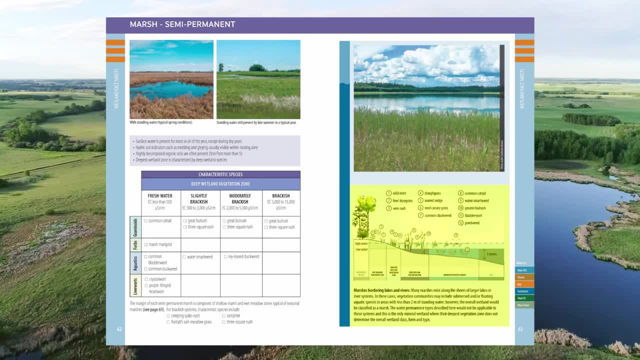 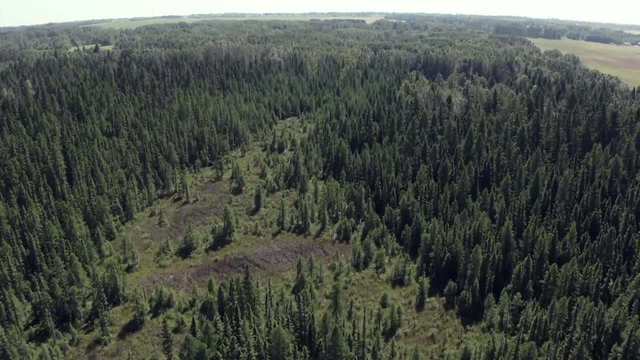 stream or river water outputs can also discharge to these downstream systems. In the boreal forest region, contiguous wetland classes connect to each other across the landscape, forming large wetland complexes. Peatlands and swamps are dominant land covers in this region.